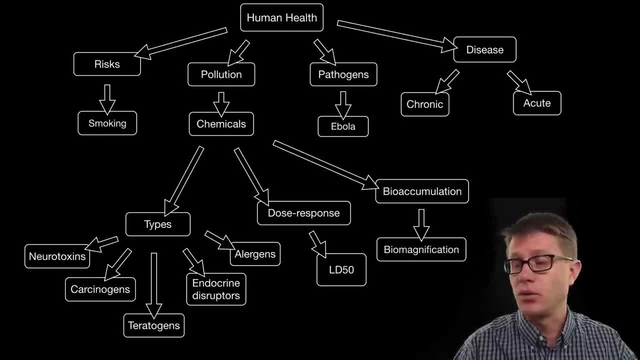 then as they move up the food chain, they biomagnify, And so we ban a lot of chemicals. The Stockholm Convention was a convention to ban 12, they called them the dirty dozen- 12 endocrine disruptors, And I think they have added another 9 since then, And so disease can be caused. 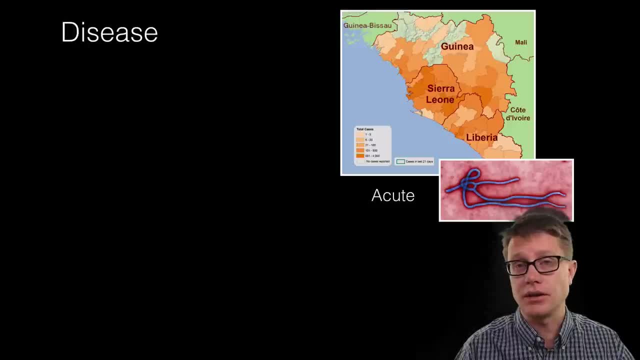 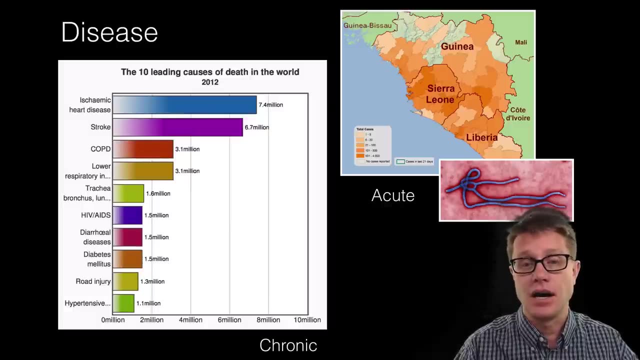 by pathogens, But they can be acute. They come on very, very quickly, Like we said, like this outbreak of Ebola recently, But most of the diseases that impact humans- so this is a list of the largest diseases in humanity- are going to come on very slowly. 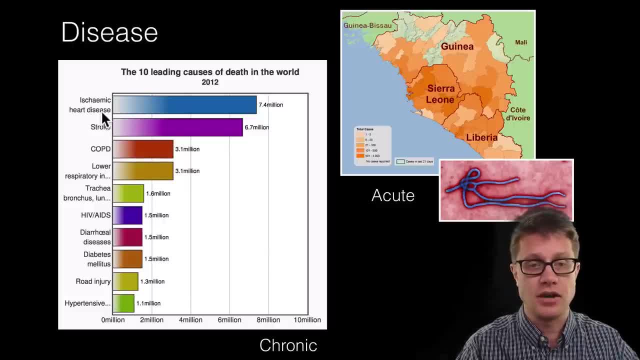 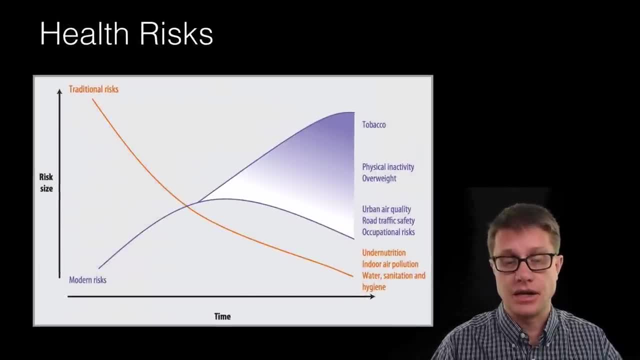 They are going to be chronic diseases of the upper respiratory tract. You see, we have heart disease, stroke, things like that that are killing most of the people on our planet. Health risks are changing over time, So it used to be that the traditional risks were. 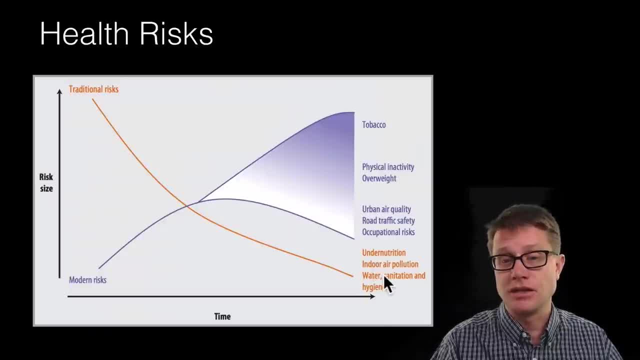 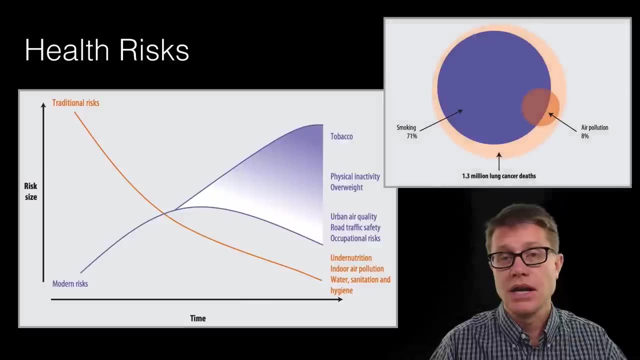 things like under nutrition, bad air pollution, inside, poor sanitation. But you can see, over time we are shifting towards more modern risks: Smoking, for example, Obesity, Inactivity, Urban air quality- These are becoming the risks of the modern world And a lot of those. 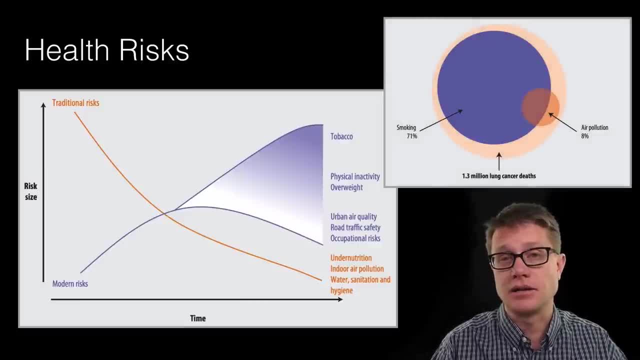 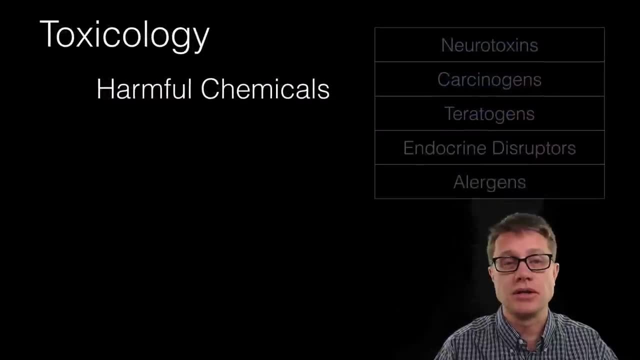 risks are ones that we take on our own. So, if we are looking at lung cancer deaths, for example, most of those are formed from smoking, Not caused by air pollution. But this video is mostly about pollution. It is about toxicology. It is about the harmful chemicals that can. 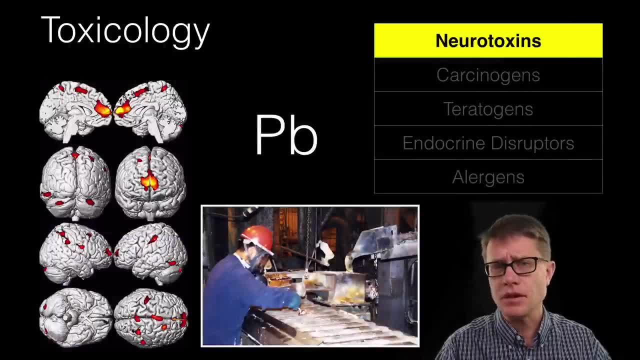 affect humans And we break those into five categories: The neurotoxins- So the methylmercury in Minamata disease would be an example of that. Lead is a great example of a neurotoxin, So it is actually damaging parts of the brain especially. 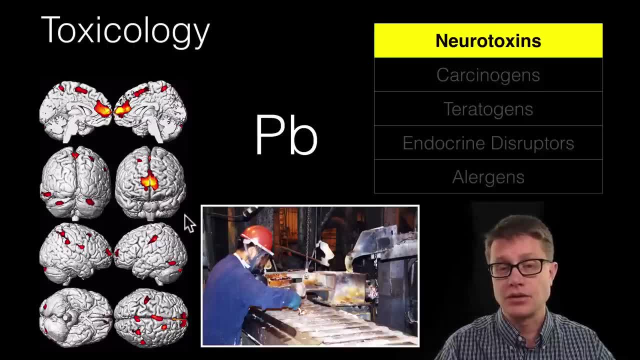 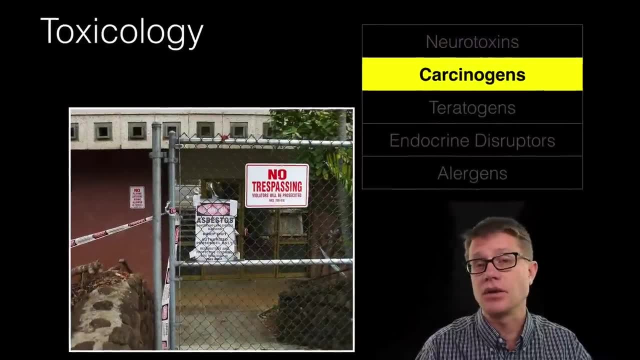 the highlighted portions here in the prefrontal cortex. So as this person right here is recycling batteries that lead, they are being exposed to lead and that is going to be a neurotoxin. We also have carcinogens. These are chemicals that can lead to cancer. A famous one would: 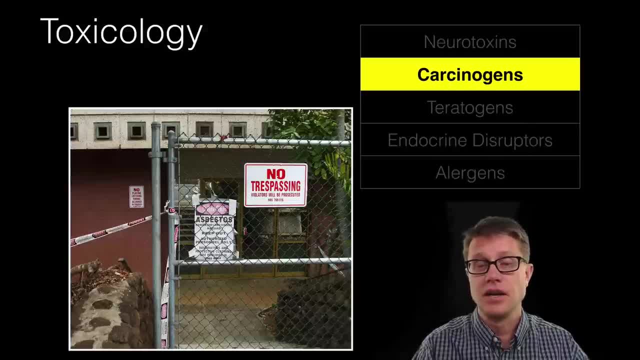 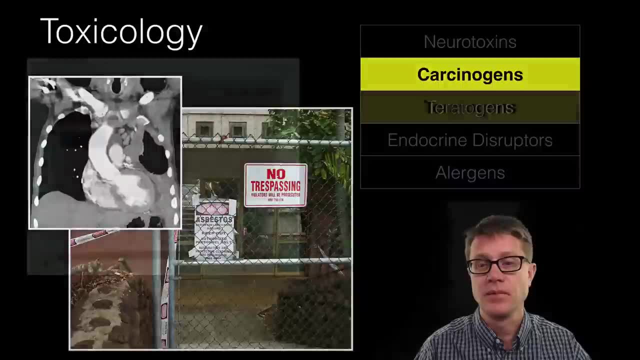 be asbestos, which was used way back in the 50's as an insulator But now causes diseases like lung cancer and mesothelioma, which is a rare form of cancer caused by asbestos. We also have teratogens. These are going to be chemicals that affect us before we are. 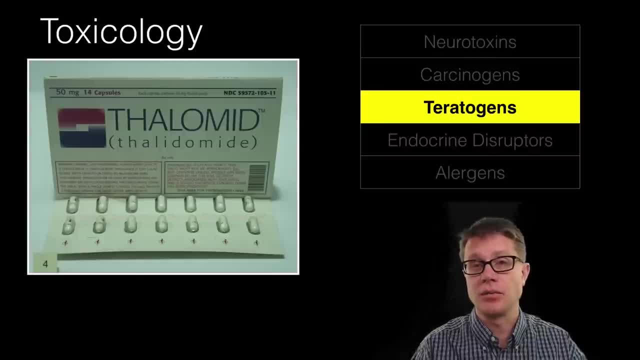 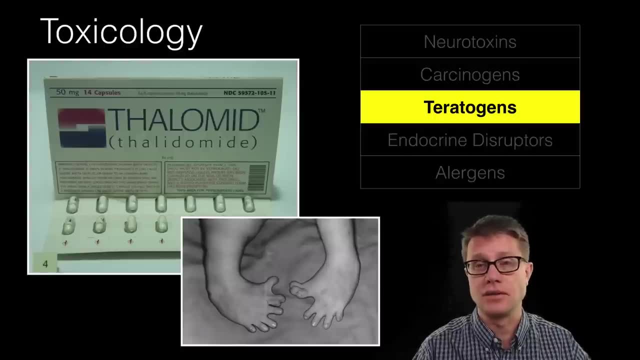 born, And so a famous example is thalidomide. It was given to women And what it does is it decreases morning sickness, But what you got were these awful birth defects, since it is a teratogen, Another example of that could be alcohol Causes fetal alcohol syndrome. 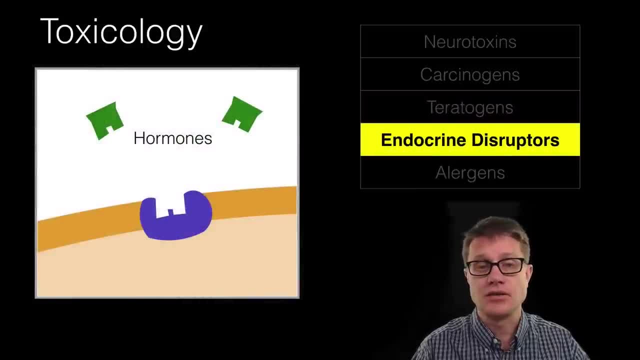 We have endocrine disruptors, And so the way that our cells communicate is through hormones. We will dock with a receptor on our cell and then there is a message that is sent into the cell. The way that endocrine disruptors work is they either block that receptor, so 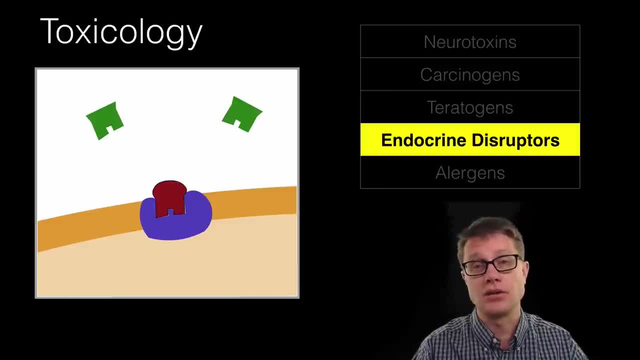 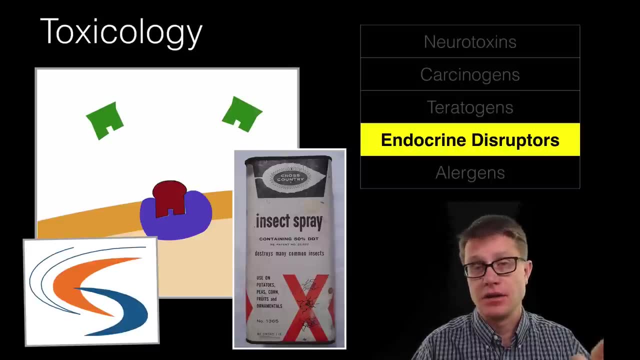 the hormone cannot dock or they can imitate the hormone itself. That is what DDT does, And the Stockholm Convention was a number of different countries that got together to ban the use of these dirty dozen, these twelve endocrine disruptors. And then, finally, we 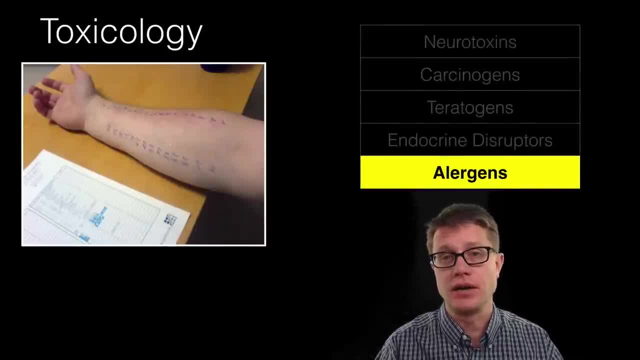 have allergens. These are going to be chemicals that affect each of us in a different way, And so this person has taken an allergy test where they are exposed to all of these drugs, So you can see that this is the result of a molecule of them, And in this case, our cell. 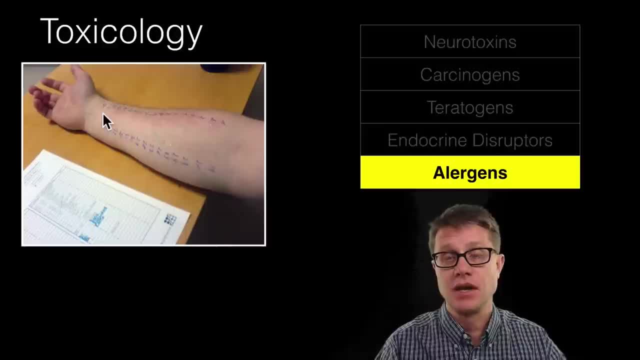 has a receptor that is going to give us the word endocrine, And so we have to stop by. and all these different chemicals, and they are seeing where the response is And this can be deadly. If you think about a peanut allergy, it can lead to anaphylaxis, And so you have. 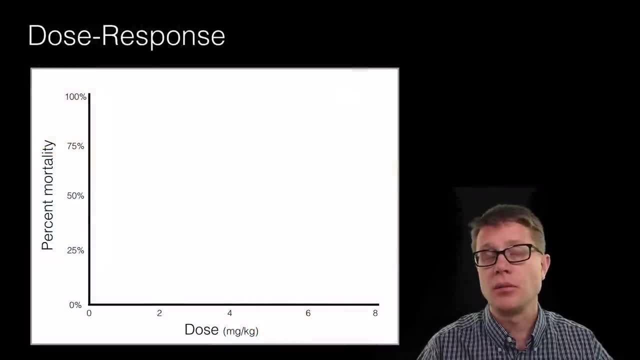 to kind of know what chemicals you are susceptible to. Now, almost all chemicals on the planet can be a toxin if we get them in large enough amounts. And so what is the safe amount of coffee, for example, that I can drink? Well, we use a test called the lethal dose or the 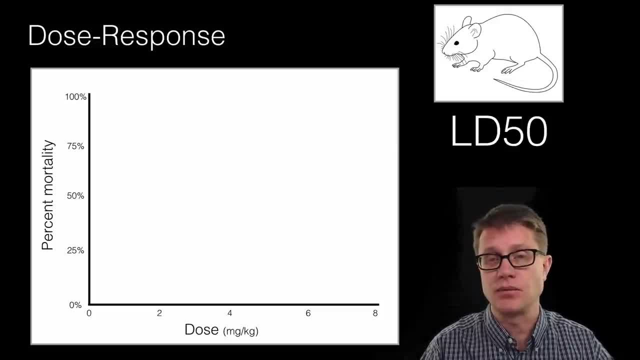 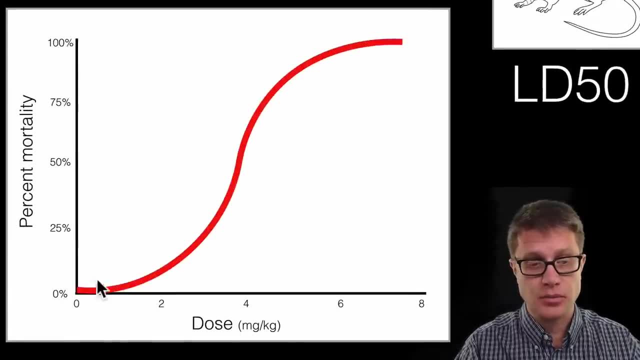 LD50 test, And a lot of this, unfortunately, is done on animals. What you do is you take a new chemical and you apply larger doses to a set of mice, for example. So the first group is giving very low amounts, low dosage, And then those at the end are giving a high. 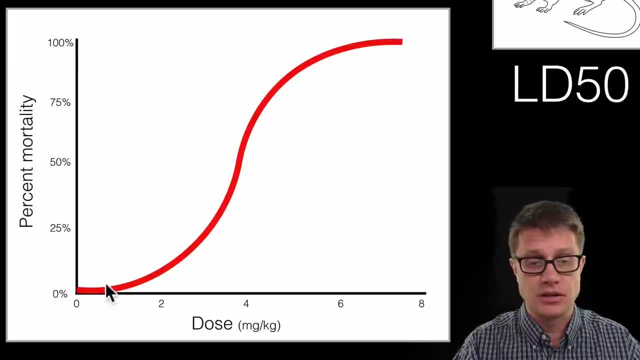 dosage And what you are looking at is mortality rate. So those that got a low dose, the percent that died is almost nil, But those who got a high dose, 100% mortality. So to calculate the LD50, what you do is you look for the point at which that graph crosses 50% mortality. 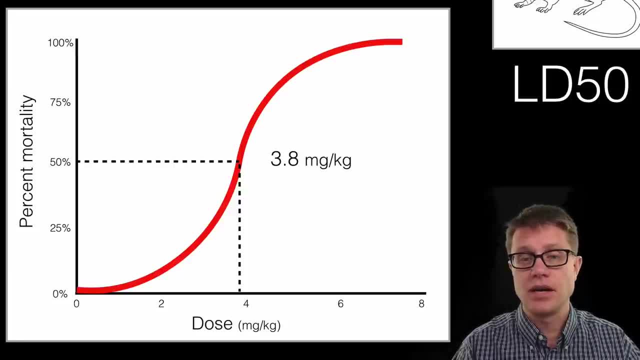 And so we could say it is at 3.8 milligrams per liter. And then you look at the LD50 and you divide that by 10. And that is going to be your LD50 for mice, And so it would be 0.38 milligrams per kilogram. That is going to be the safe dose, If we see where that. 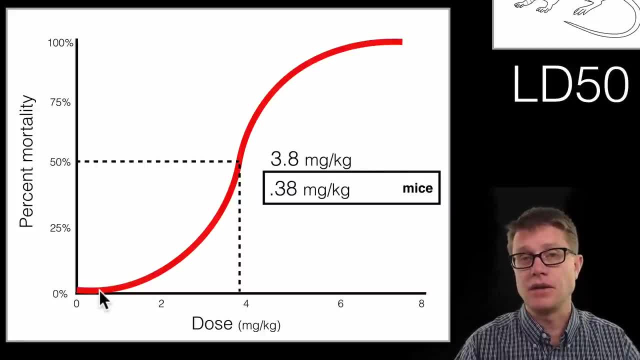 is on the graph. it is going to be way down here Now the LD50. then to extrapolate that for humans, what we will do is we divide it by 10 again, Because there may be different susceptibility in humans and mice, And then we will divide it by 10 again, just to be safe. 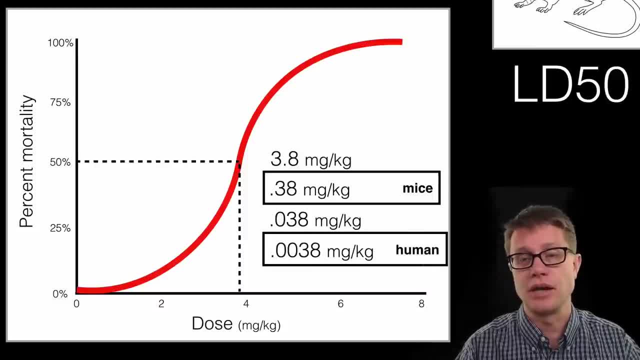 And so the LD50 in humans would be 0.0038 milligrams per kilogram. And then you divide that by 10. And that is going to be 1.8 milligrams per kilogram. Now the problem with a lot. 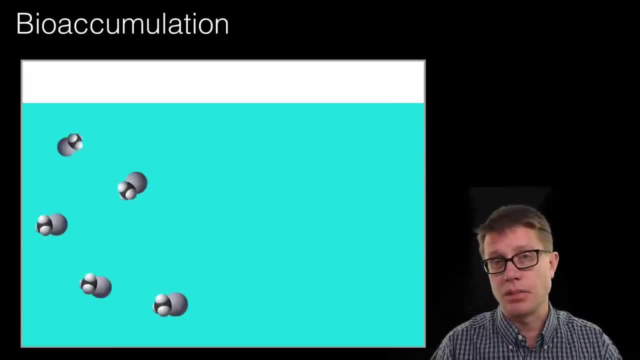 of these chemicals is they bioaccumulate. So that methylmercury that was pumped into Minamata Bay was picked up by phytoplankton. In other words, as they were taking in water, they are taking some of those chemicals. They do not kill those phytoplankton, But those phytoplankton are eaten by zooplankton, which are eaten by small fish. And as we move up the food chain, the chemicals do not go away. They bioaccumulate, And so over time they get to larger and larger doses, And so the EPA put a list out of what they were eating. 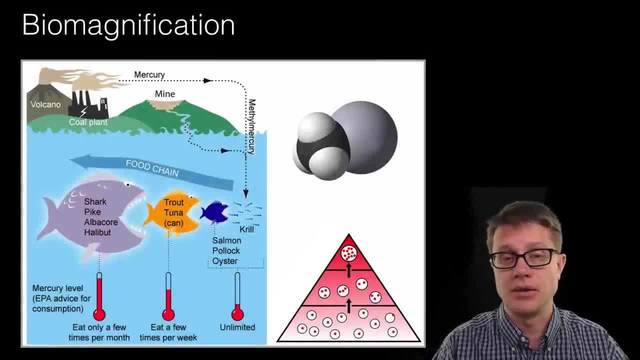 Of what fish are safe to eat in an area where methylmercury may be found. And so they said that at the lower parts of the food chain- krill and maybe oysters, for example- it is safe to eat an unlimited amount of these, But as we move up to tuna and sharks, you should. 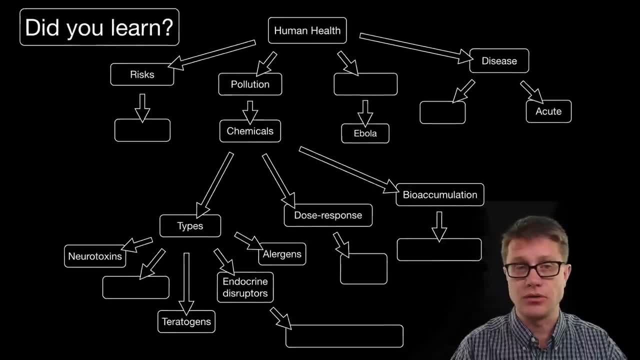 minimize the amount that you are eating, because there are going to be larger loads of mercury. Did you learn the following? Could you pause the video at this point and fill in the blanks? Let me do that for you. Human health can be impacted by diseases which are chronic. it 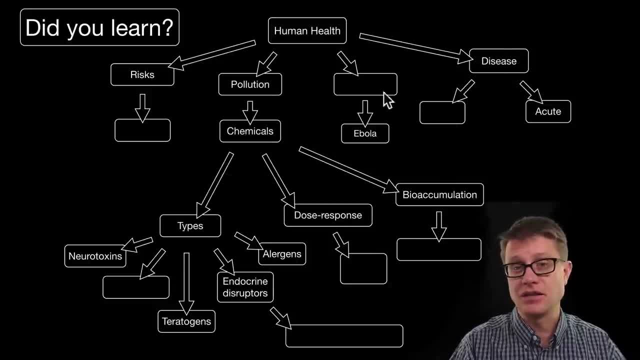 takes a long time or acute, Can be caused by pathogens like viruses, for example Ebola virus, Or risks like smoking. But pollution is chemicals that are toxic to us. We break those into five categories: Neurotoxins, carcinogens, teratogens, endocrine disruptors. Remember we used the Stockholm? 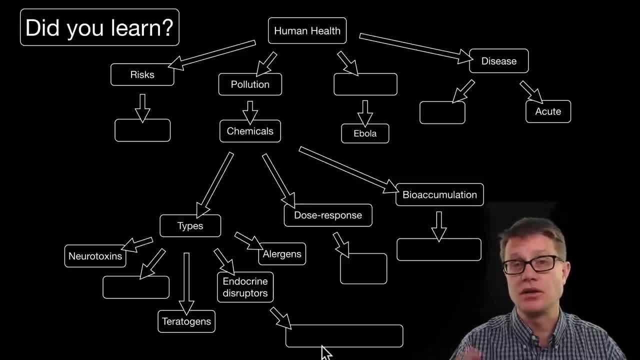 Convention as a treaty to try to stop using the dirty dozen of these endocrine disruptors. We have allergens which affect each of us differently. The dose response we use is the LD50 test, And then the thing that we have to be wary of in environments is that we have 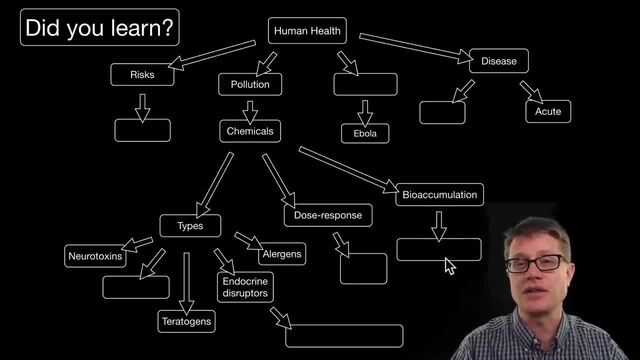 bioaccumulation, biomagnification, That is, health impacts of pollution, And I hope that was helpful. 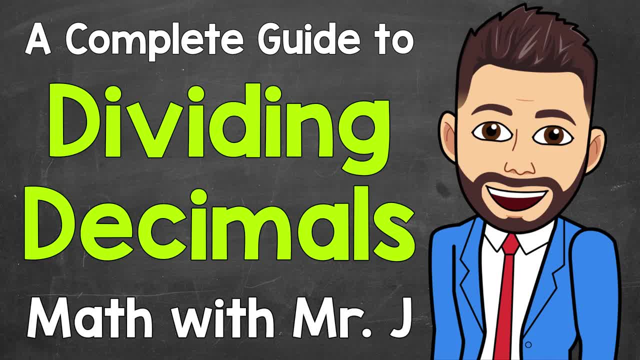 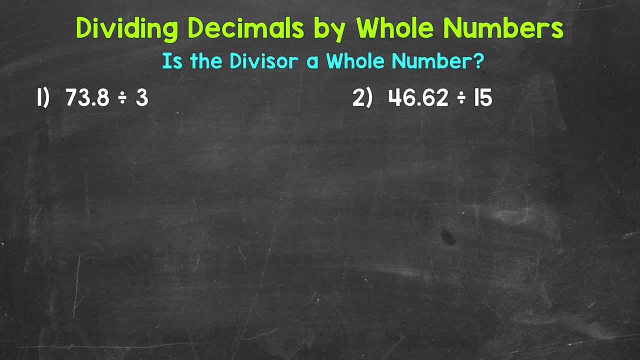 Welcome to Math with Mr J. In this video I'm going to cover division involving decimals. This is going to be a complete guide to dividing decimals. I'll cover dividing decimals by whole numbers, whole numbers by decimals, decimals by decimals and dividing by mixed decimals.